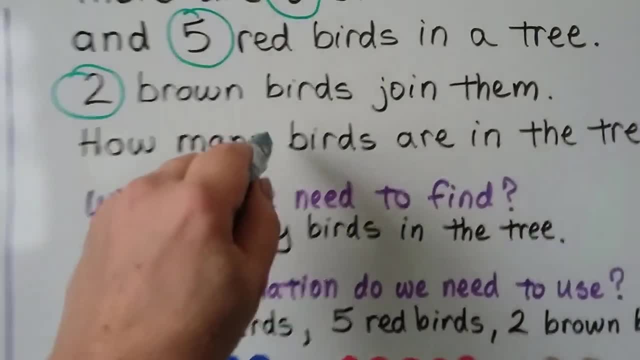 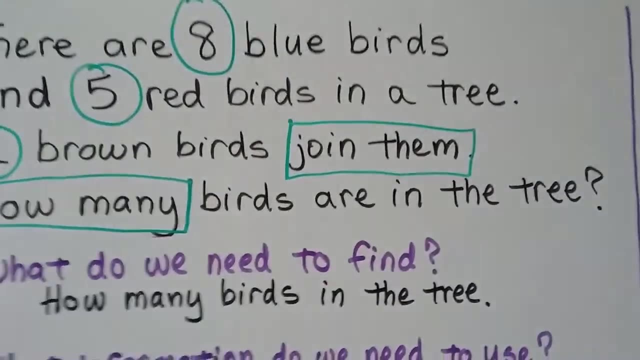 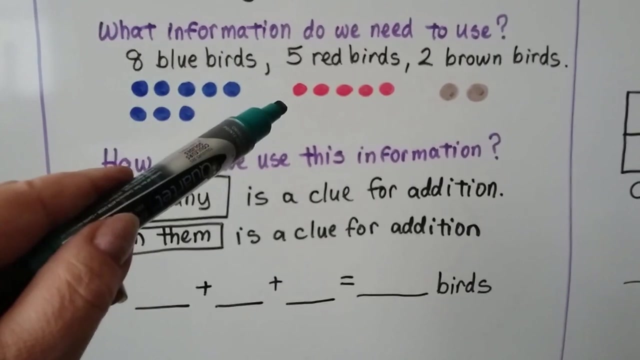 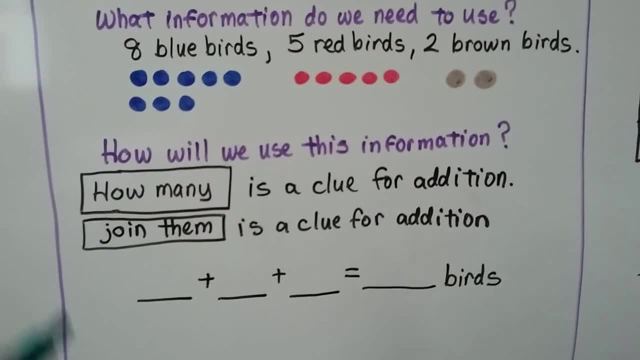 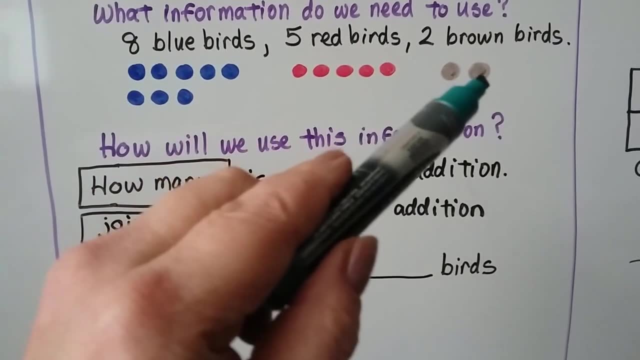 and two brown dots for the brownbirds. We can count them Eight, nine, ten, 11,, 12,, 13,, 14,, 15,, 16,, 17,, 18,, 19,, 20,, 21,, 22,, 23,, 24,, 25,, 26,, 27,, 28,, 29,, 30,, 31,, 32,, 33,, 32,. 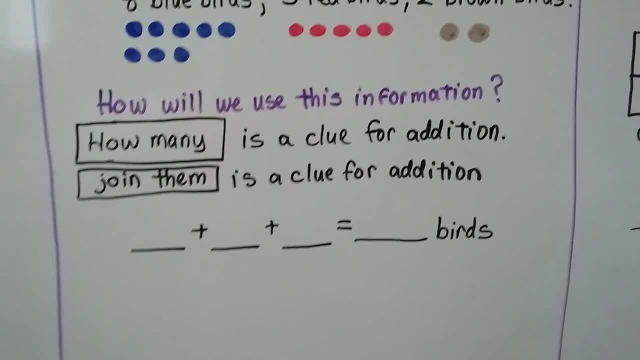 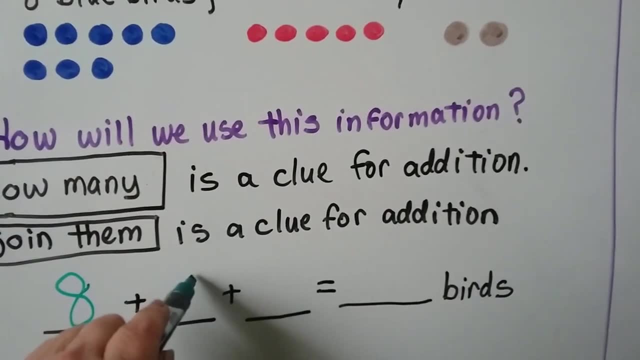 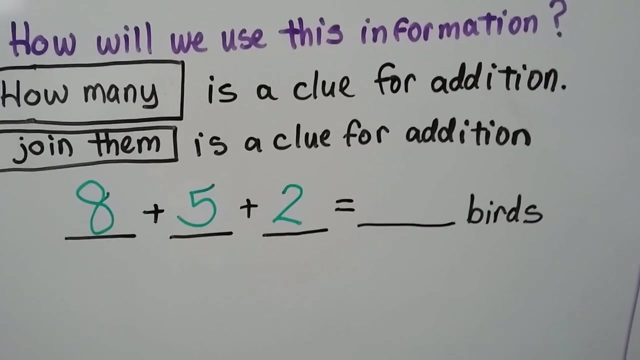 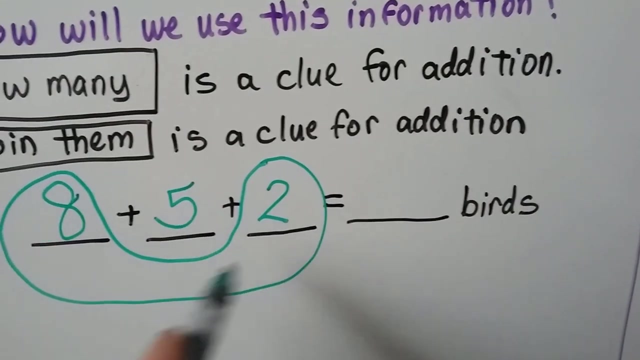 We can write an addition sentence 8 would be the first addend, 5 would be the next addend and 2 would be the last addend. We can make a 10.. We could take this 2 and this 8 together. 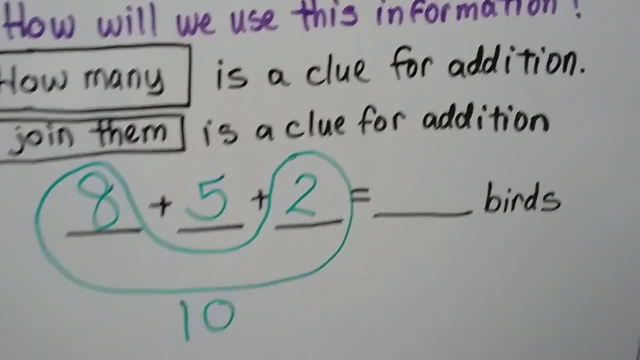 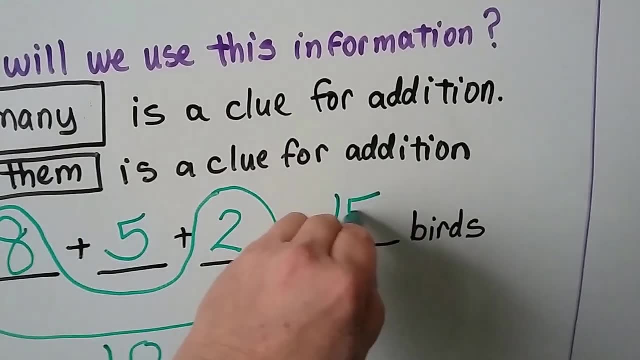 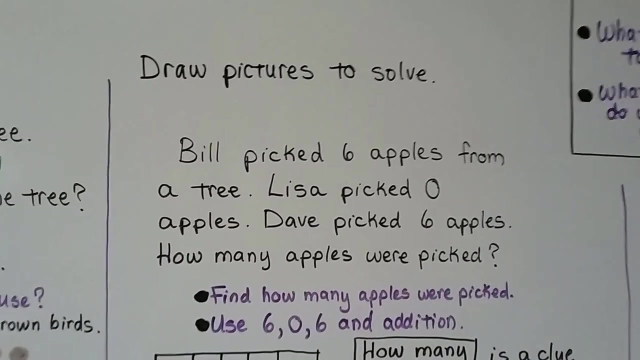 and make a 10 and then add the 5. 10,, 11,, 12,, 13,, 14,, 15.. 15 birds are in the tree. We can draw pictures to solve. Bill picked 6 apples from a tree. Lisa picked 0 apples. 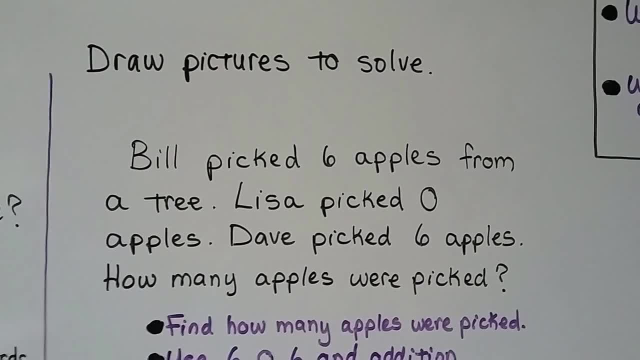 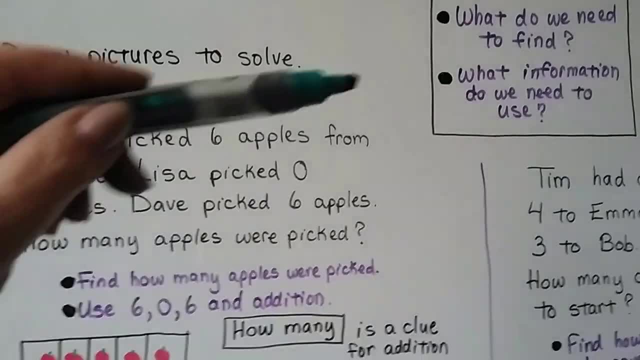 Dave picked 6 apples. How many apples were picked? What do we need to solve this problem? What do we need to solve this problem? What do we need to solve this problem? We need to find. We need to find how many apples were picked. What information do we? 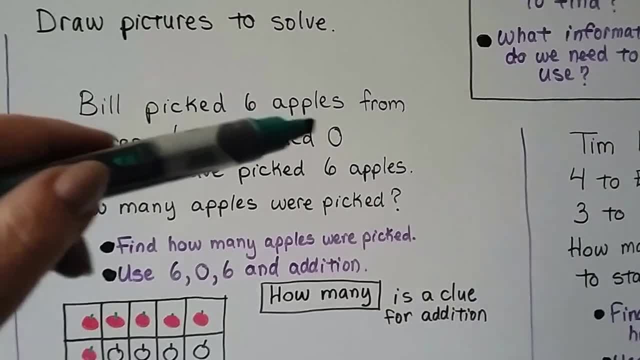 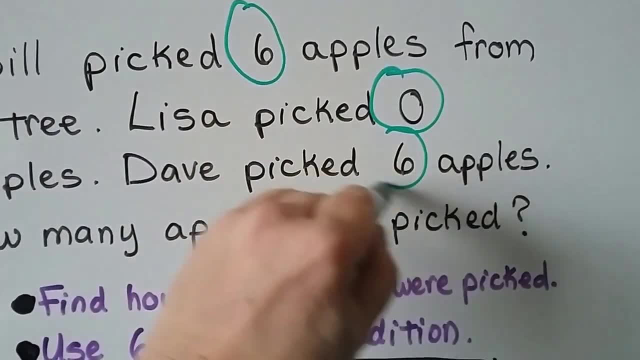 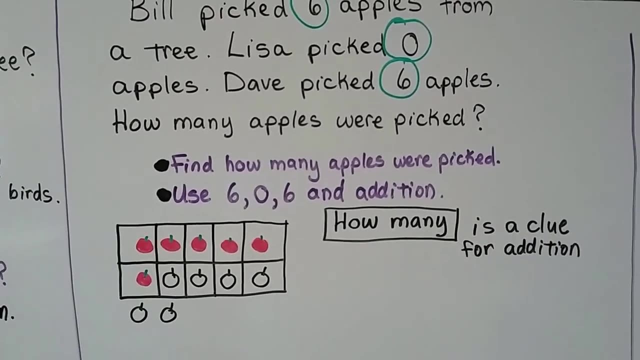 need to use? We need to use the 6,, the 0, and the 6.. Those are the important numbers in the problem. How will we use the information? How many is a clue. for addition, It's asking how many were picked. 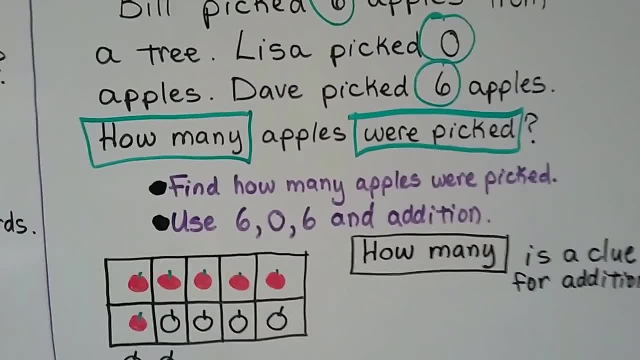 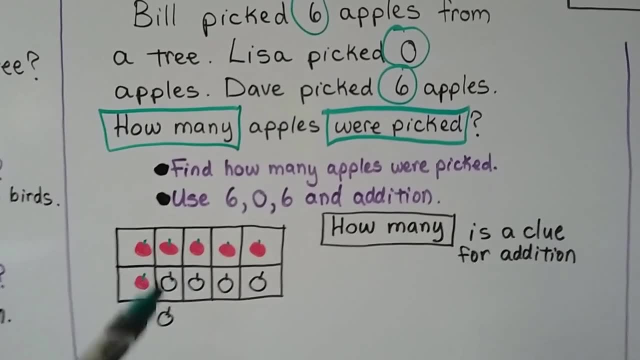 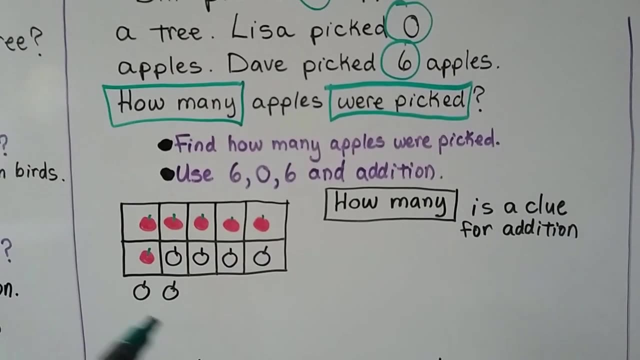 That tells us we need to add the numbers. We can make 6 apples for Bill's Lisa is 0, so we put 0 for Lisa and Dave picked 6.. We can fill the 10 frame with 4 of them and 2 are outside. Now we know there's 10,, 11,, 12.. 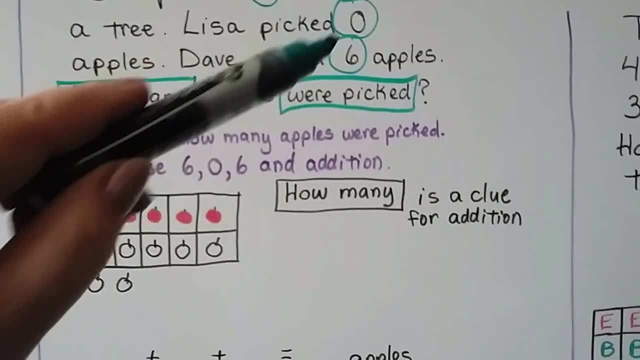 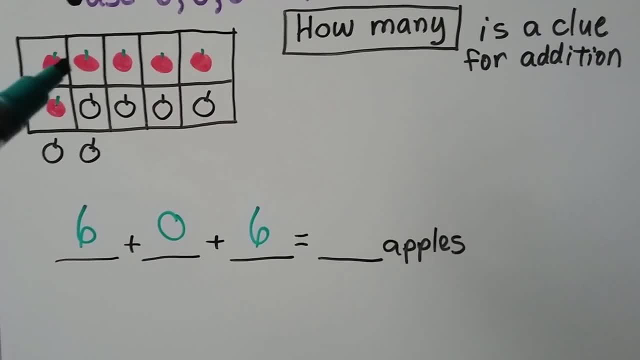 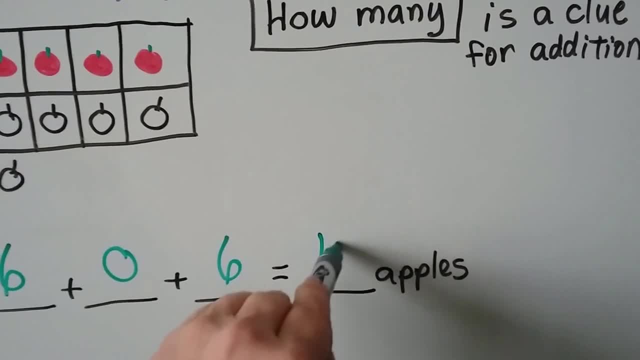 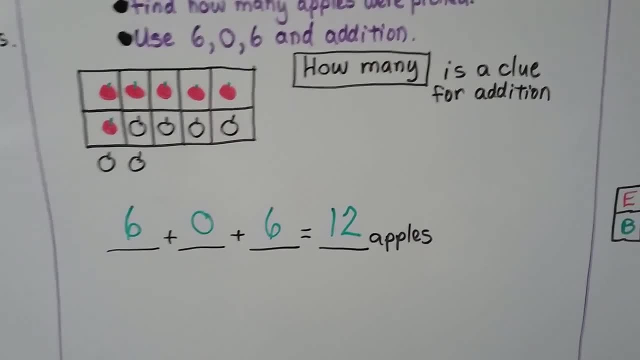 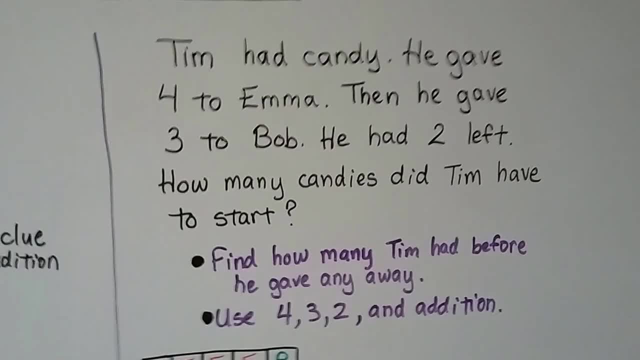 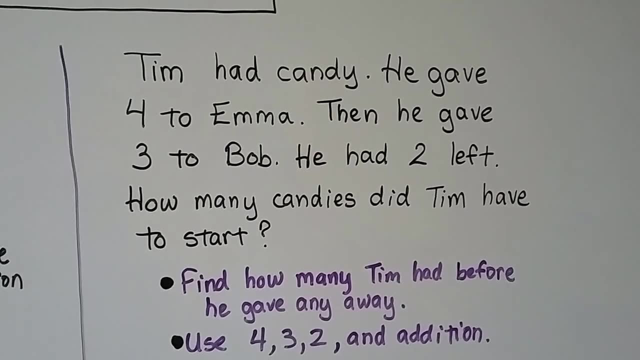 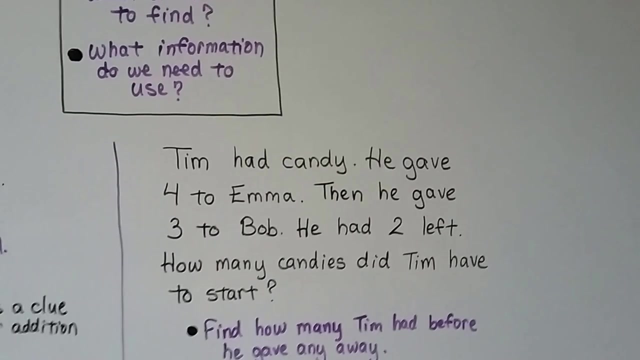 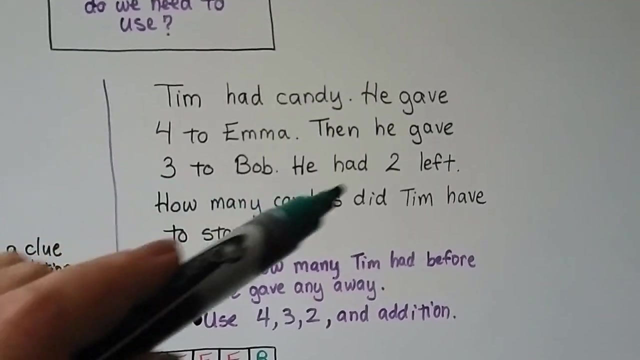 Tim had candy. He gave four to Emma, then he gave three to Bob. He had two left. How many candies did Tim have to start? So what do we need to find? We need to find how many Tim had before he gave any away. And what information do we need to use? We need to use the four, the three and the two. 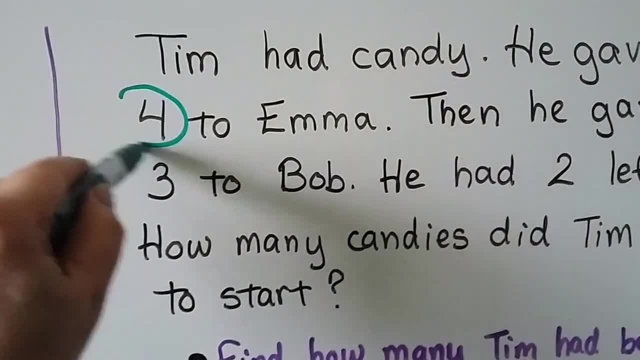 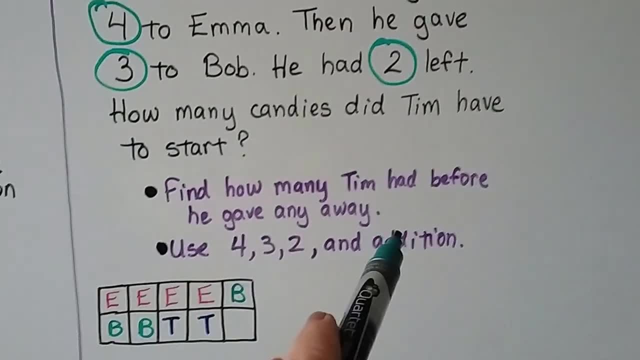 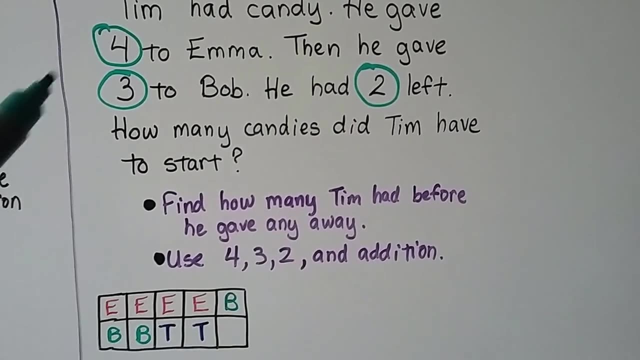 and addition. These are important numbers: the four, the three and the two. How will we use the information? We'll use addition. It's asking how many. What we can do is make a 10 frame and he gave four to Emma. Emma starts with an E. 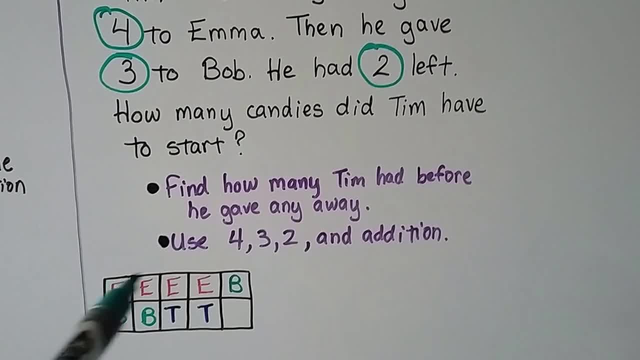 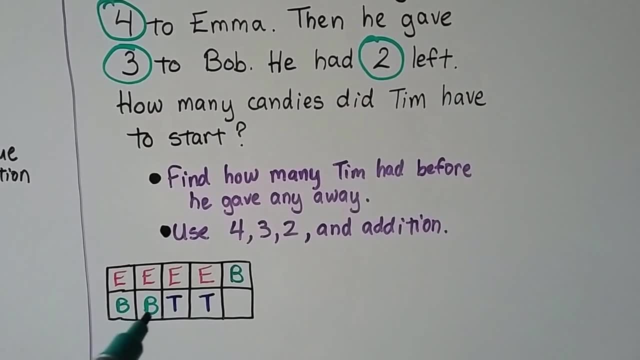 so we can make one, two, three, four E's for Emma's for her four. He gave three to Bob. We can make a B, A, B for Bob and another one and another one to make the three to Bob, And he had two left. 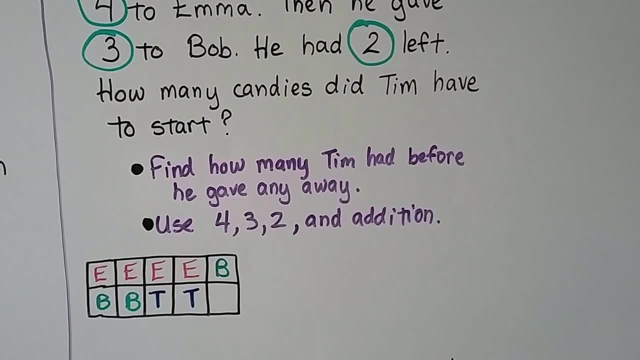 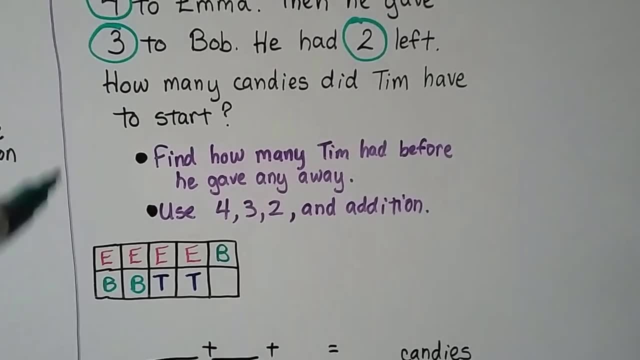 and his name is Tim, so we can put one, two T's for Tim. We can look at the 10 frame and see that it's one less than 10.. It's nine And we can use the four, the three and the two to write an. 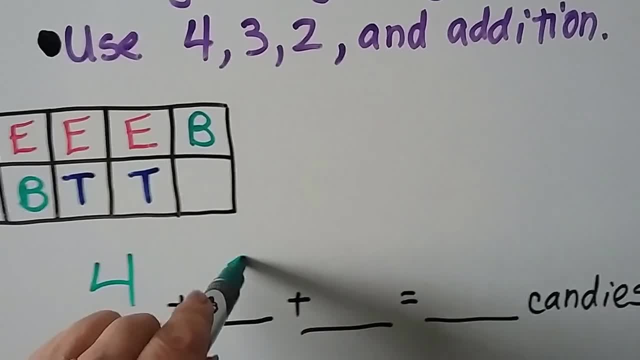 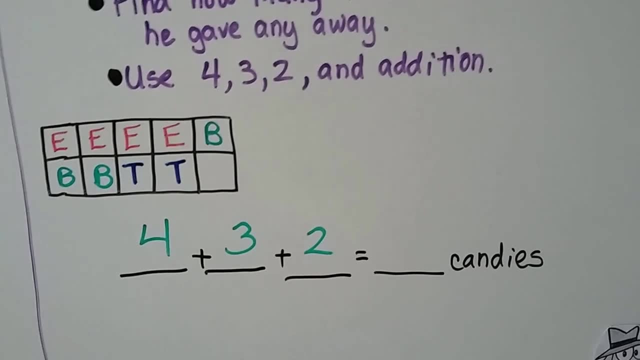 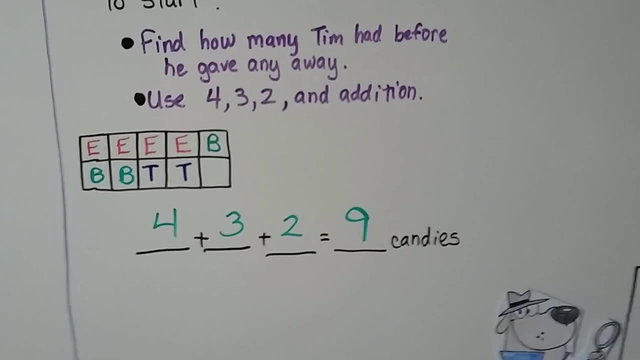 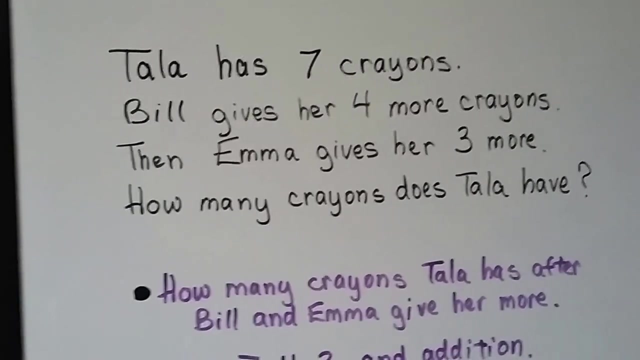 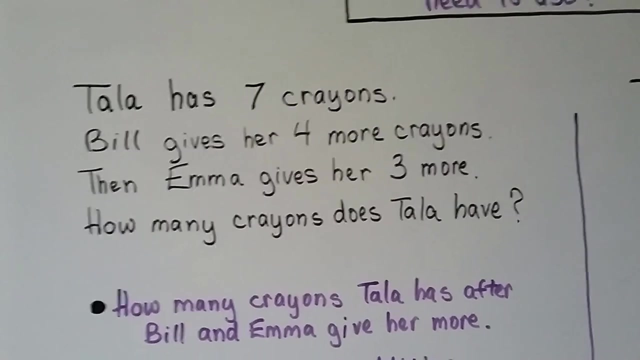 addition, sentence Four and three and two, And we can see from our picture that he had nine candies to start. Tala has seven crayons. Bill gives her four more crayons, Then Emma gives her three more. How many crayons does Tala have? What do we need to find? We need to find how many crayons Tala has. 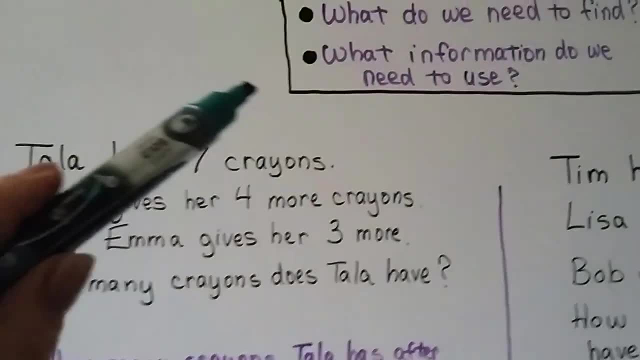 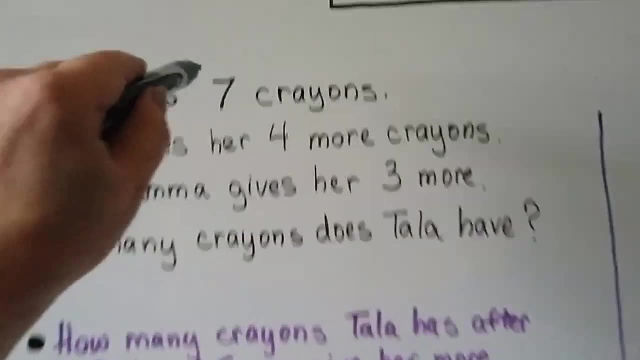 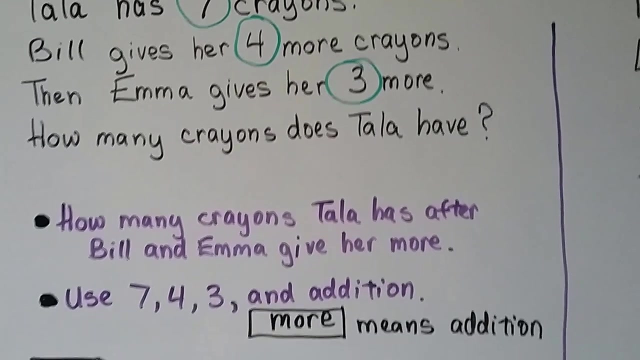 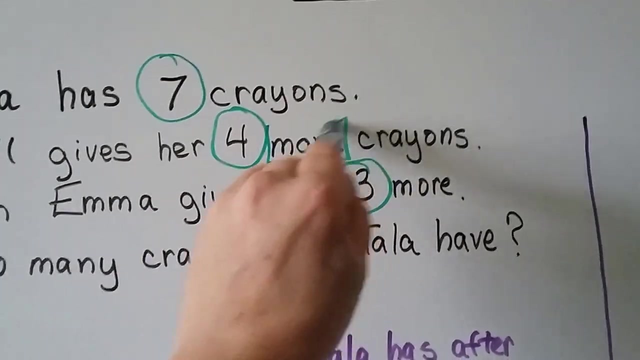 after Bill and Emma give her more. What information do we need to use? We need to use the seven, the four and the three. These are the important numbers: seven, four and three. How will we use the information? Addition, More means addition. We see that Bill gives her more, Emma gives her more. 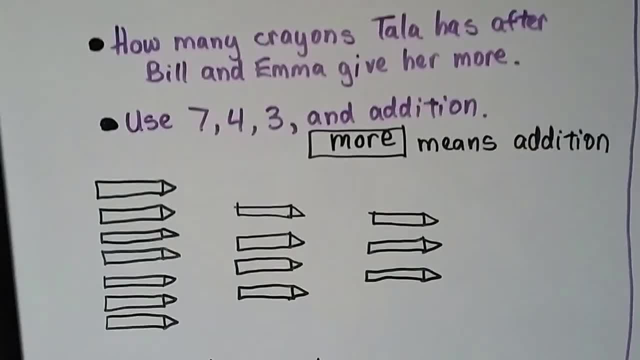 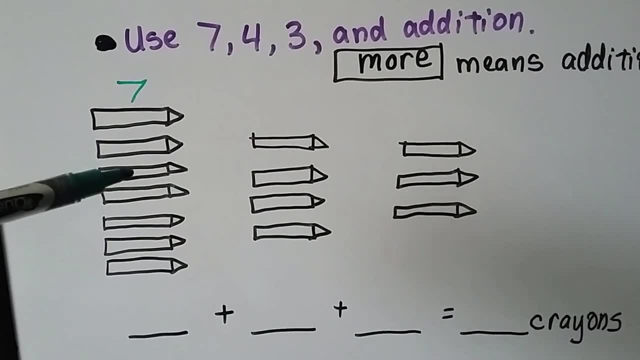 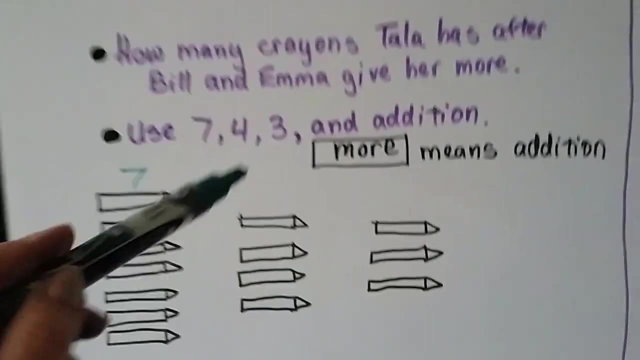 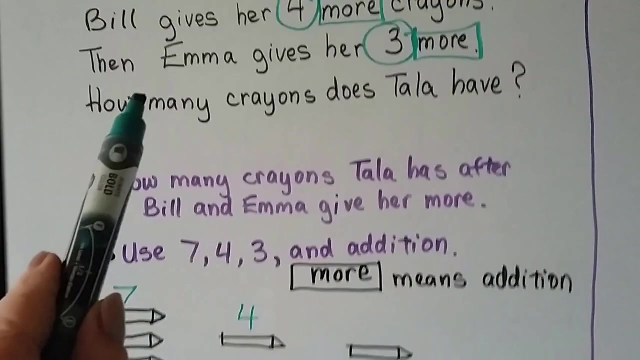 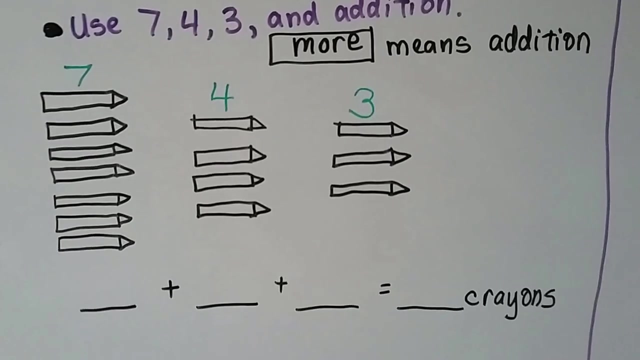 So we're going to add these numbers. We can draw a crayon. here's the seven that she had: one, two, three, four, five, six, seven. we can draw seven simple crayons. here's the four. bill gives her four more, so these are four from bill, and Emma gives her three more, so here's the three from Emma. we 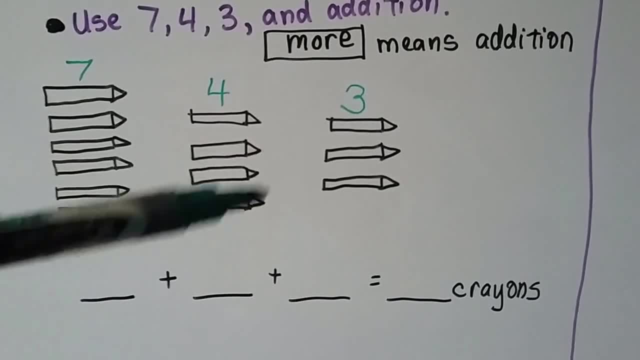 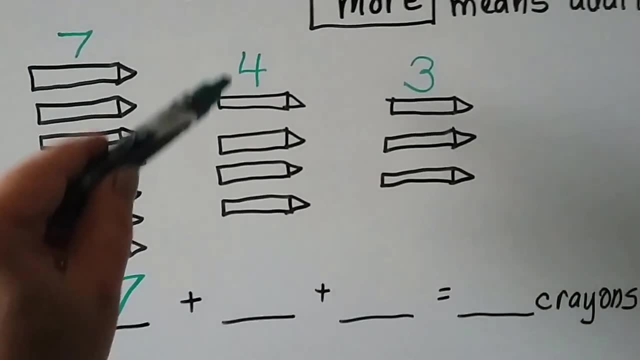 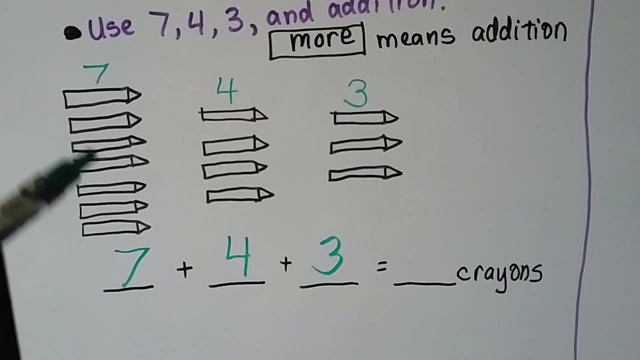 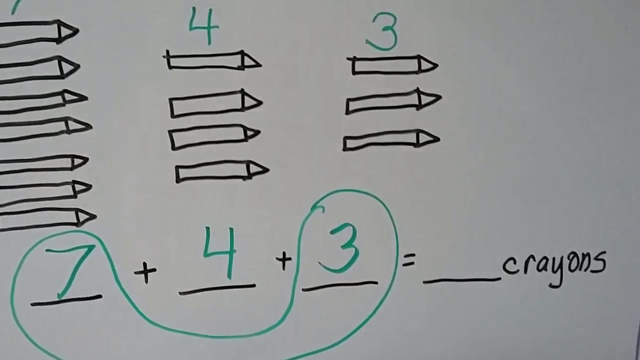 can add seven, eight, nine, ten, eleven, twelve, thirteen, fourteen. we can write an addition sentence: seven plus four plus three, and we can add them: seven plus three would make a ten. we could take these two add-ins together and make a ten right, seven plus three. then we can add the: 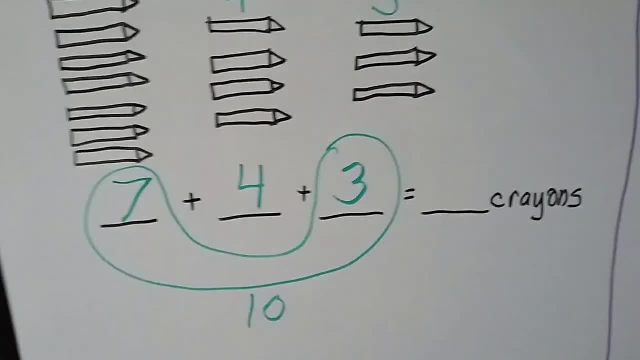 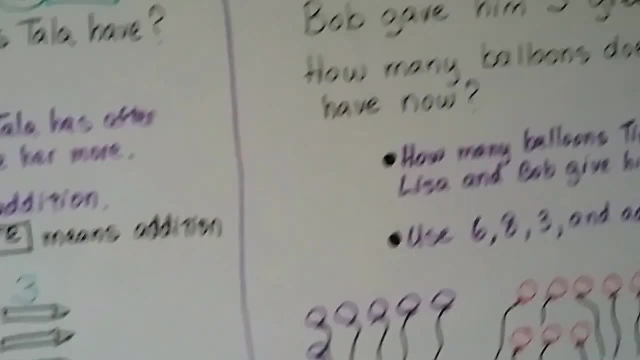 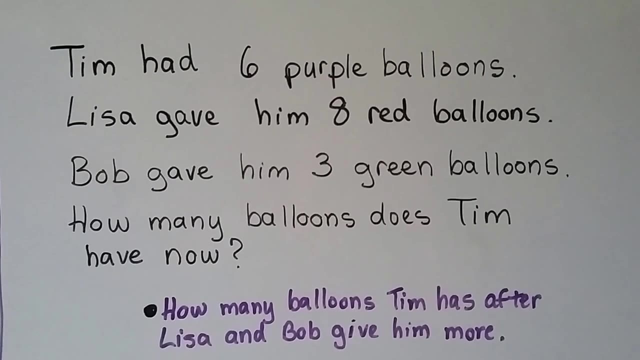 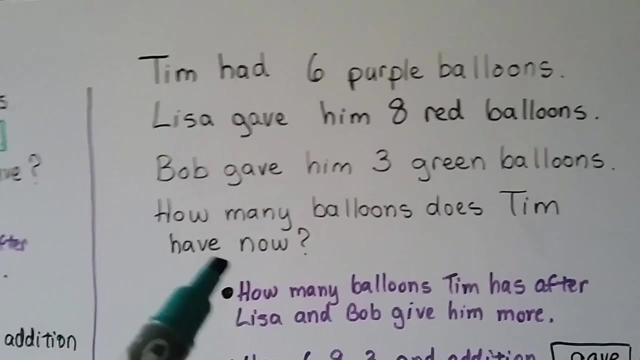 four, ten, eleven, twelve, thirteen, fourteen, so now she has 14 crayons. Tim had six purple balloons, Lisa gave him eight red balloons. Bob gave him three green balloons. how many balloons does Tim have now? what information do we need to find how many balloons Tim has after Lisa and Bob give him more? what information?